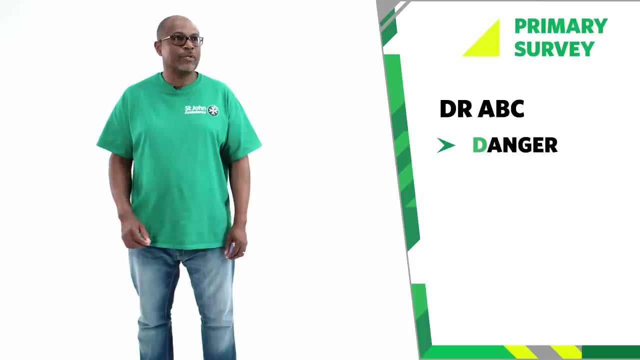 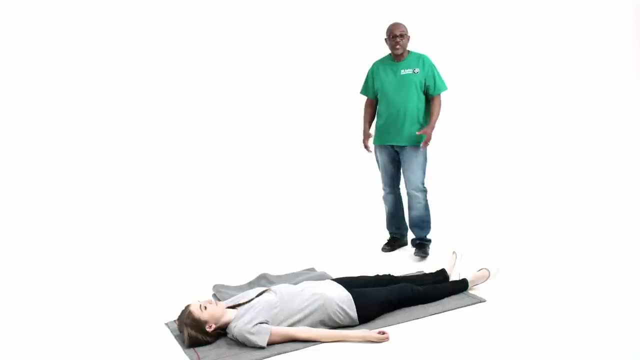 These initials stand for Danger Response, Airway Breathing and Circulation. So when I see a casualty, first I'm going to check for any danger, to make sure it's safe for me to approach them. I don't want to become a casualty myself. 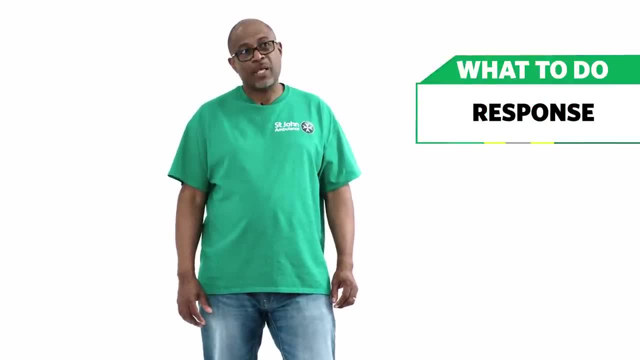 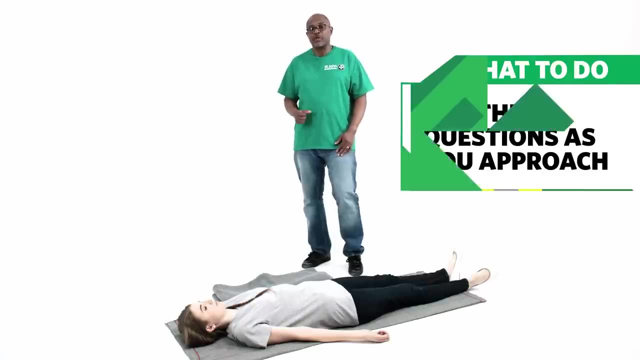 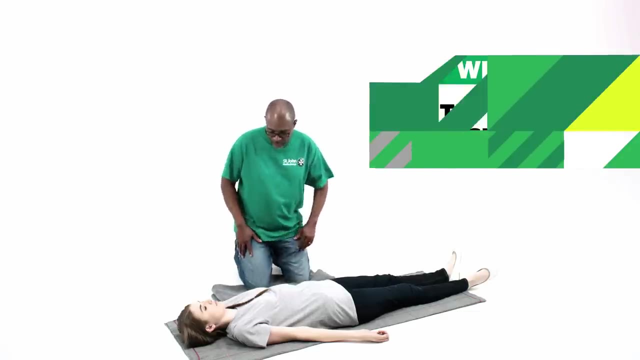 Then I'm going to see if I can get a response from the casualty. As you approach, introduce yourself, Ask them questions to try to get a response. If they're not alert and do not respond to your voice, kneel down beside them and gently shake their shoulders. 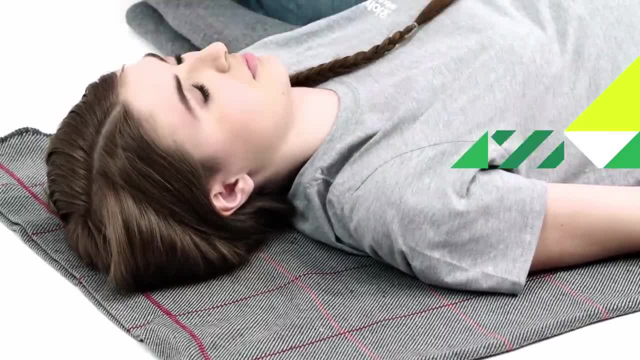 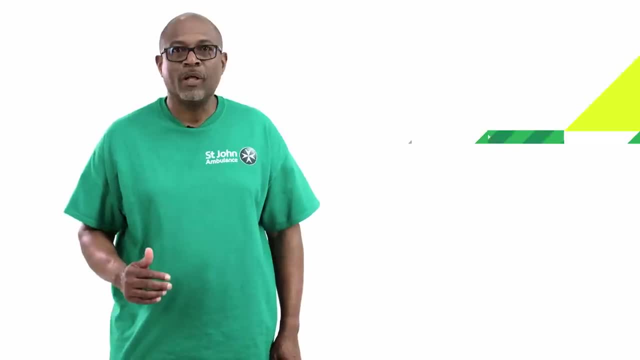 Hello Amy, it's Winston. Can you hear me Open your eyes? Still no response. You can pinch their earlobe to see if they respond to pain. Depending on how the casualty responds to you, we'll establish a level of response. 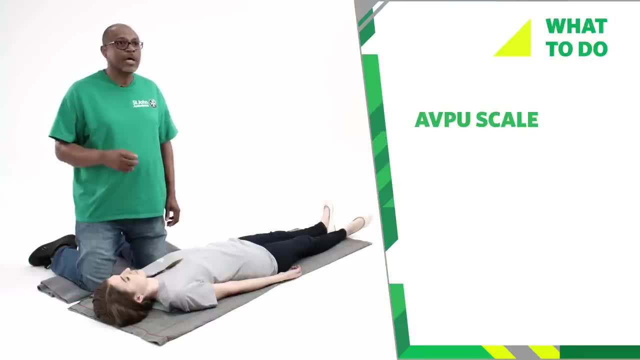 We use the AVPU scale and each letter can represent the casualty's level of response: A alert: V response to voice, P response to pain And U is the casualty unresponsive to stimuli. If there's still no response, they're unresponsive. 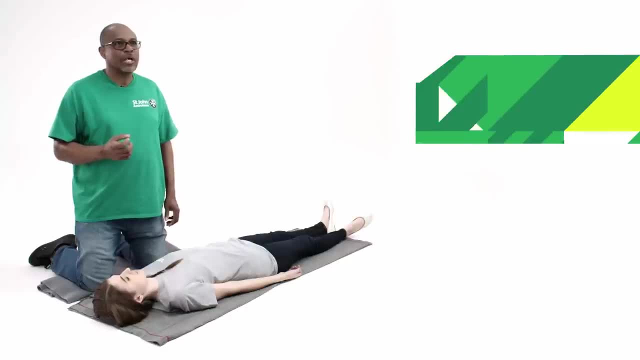 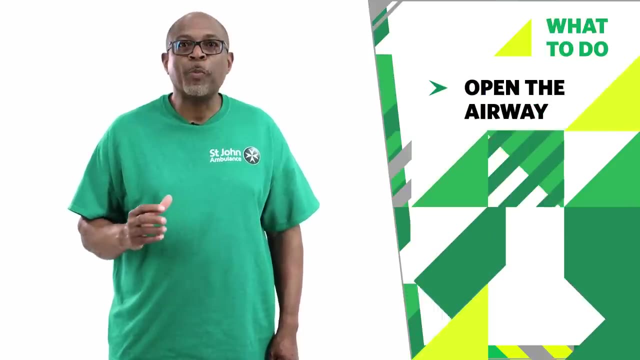 We need to check the airway Is the casualty alert- and speaking to you, You know that there's no problem with the airway. It is clear. If the casualty is unresponsive, open the airway by putting one hand on the forehead and gently tilting the head back. 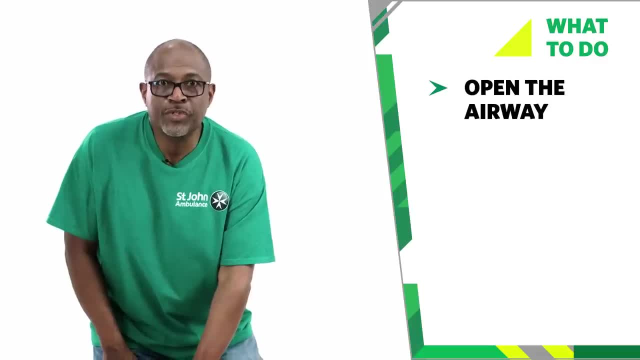 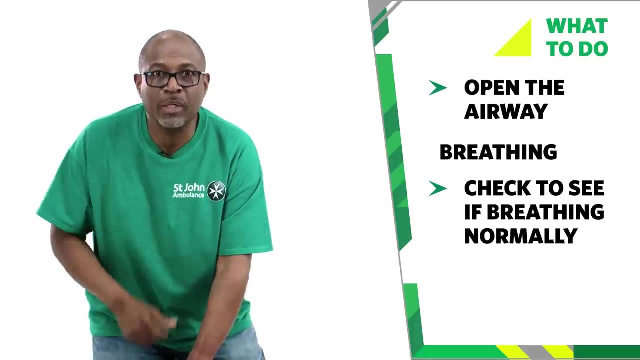 With two fingers under the chin. Now we need to check to see if they are breathing normally. We do this by placing our ear and cheek over their nose and mouth, looking down the body to see if the chest rises and falls. We do this for 10 seconds. 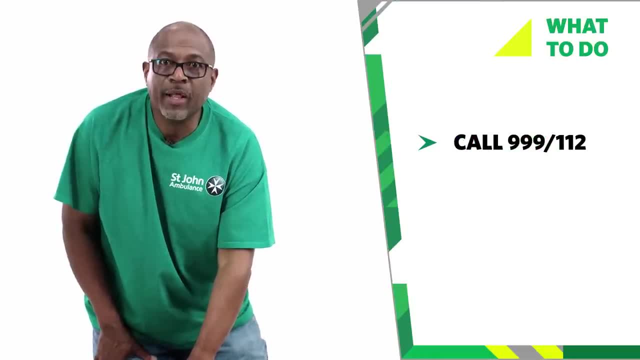 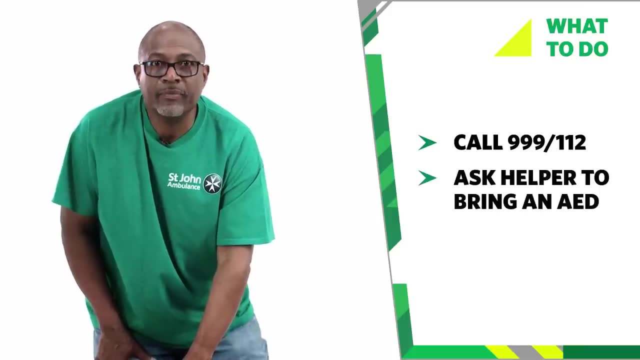 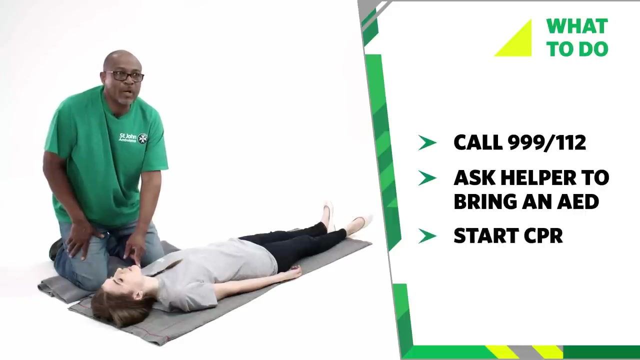 If the casualty is not breathing normally, call for help. Ask them to call 999 or 112 for emergency help and bring an AED. If you are alone, call for emergency help using a mobile or speakerphone and begin CPR with chest compressions.